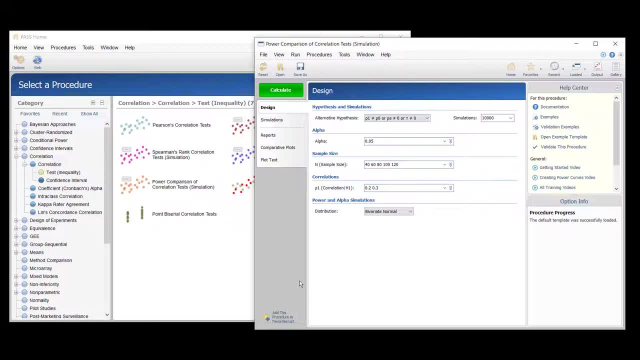 correlation test and Kendall's tau correlation test. These last two tests are nonparametric tests. Suppose a study will be run to test whether the correlation between forced vital capacity X and forced expiratory value Y in a particular population is nonzero. Researchers wish to find the power if 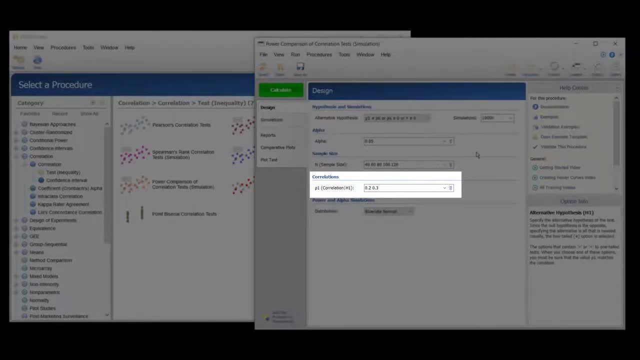 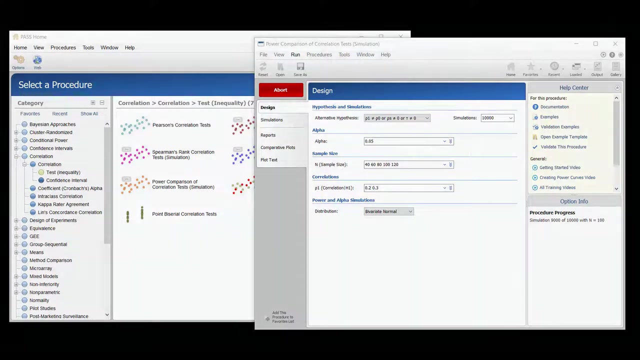 the underlying correlation is 0.2 or 0.3, alpha is 0.05 and for sample sizes of 40,, 60,, 80,, 100 and 120.. The first power comparison is made with the assumption of a bivariate normal distribution For underlying correlations of both 0.2 and 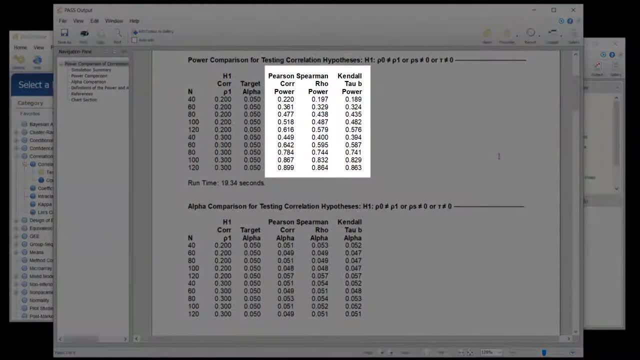 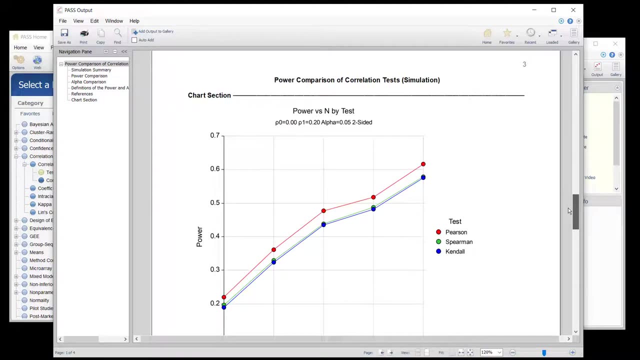 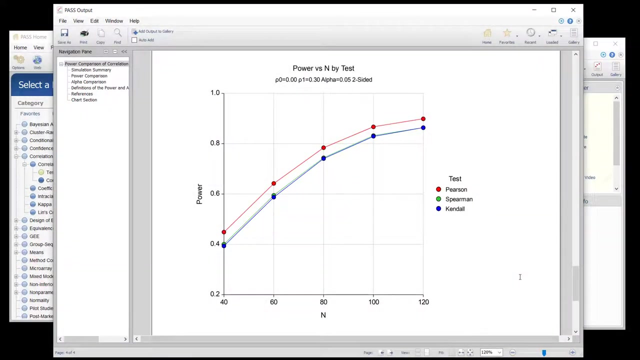 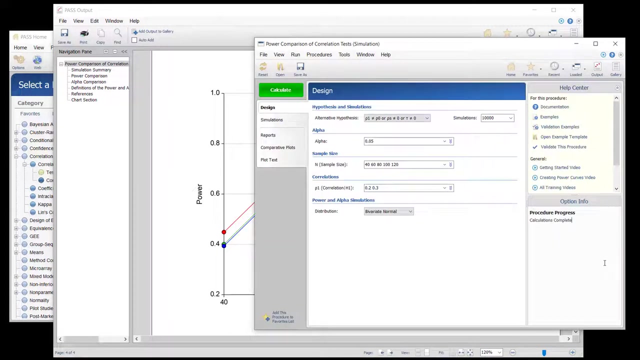 0.3,, alpha is 0.05 and for sample sizes of 40,, 60,, 80,, 100 and 120.. The first power Three, the Pearson test, has a higher power. A second power comparison is made with the same assumed correlations but where a custom. 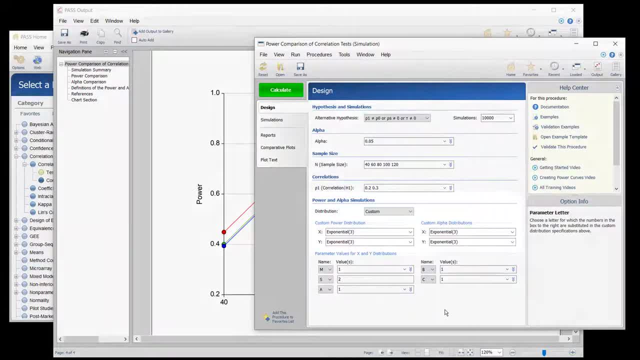 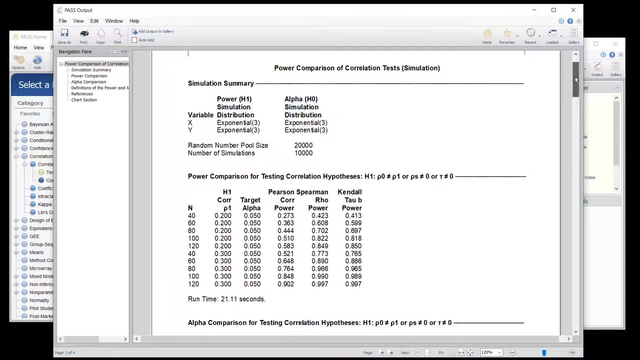 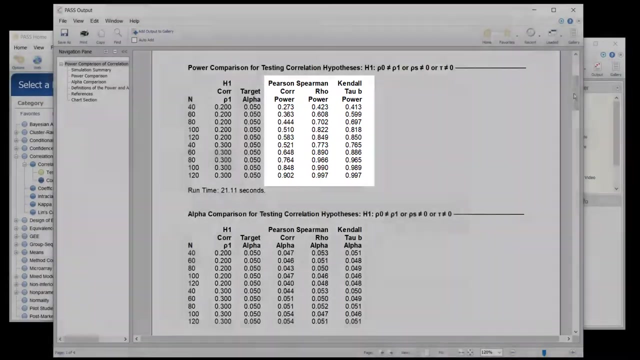 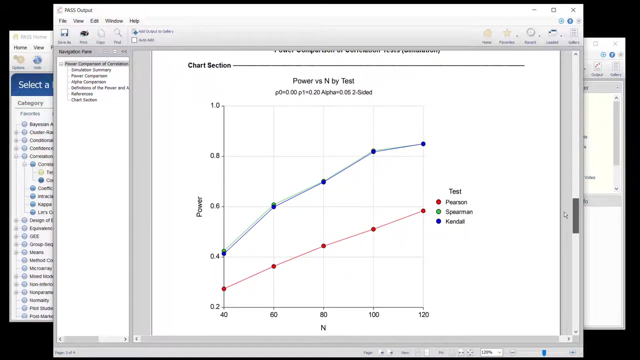 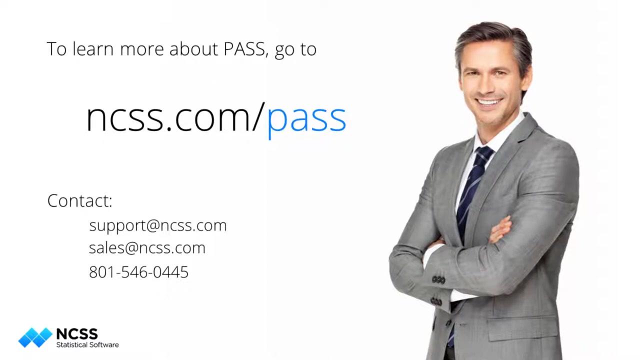 bivariate distribution is assumed with exponential marginal distributions. In this case, the two non-parametric tests have much higher power. To learn more about this sample size procedure or the hundreds of other sample size tools in PASS, see the help documentation that is installed with the software and is also available. 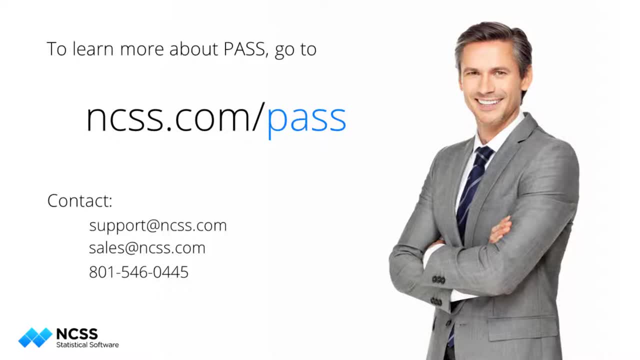 online at ncsscom. If you are new to PASS and would like to learn more about it, you can download the free trial.